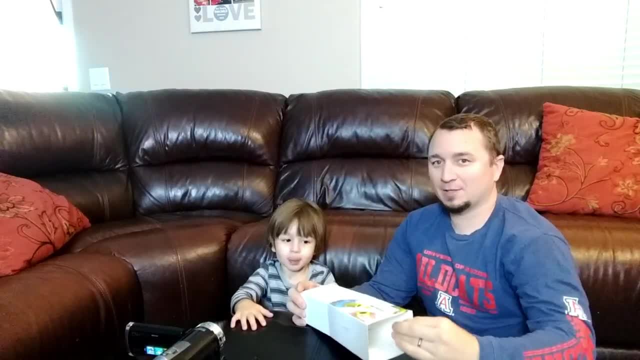 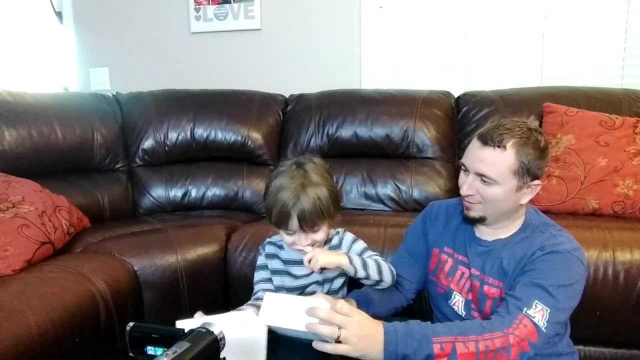 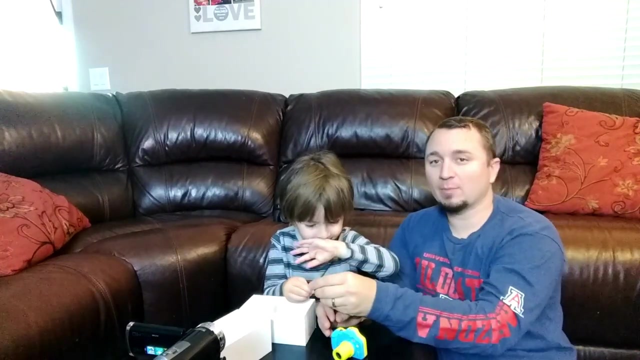 Here. let's see, let's push it open. You can see he likes having cameras and recording himself. Whoa Tiny, This is tiny. huh, Oh, look a Nami car. So this camera doesn't come with a memory card, but we're going to use a micro SD card. 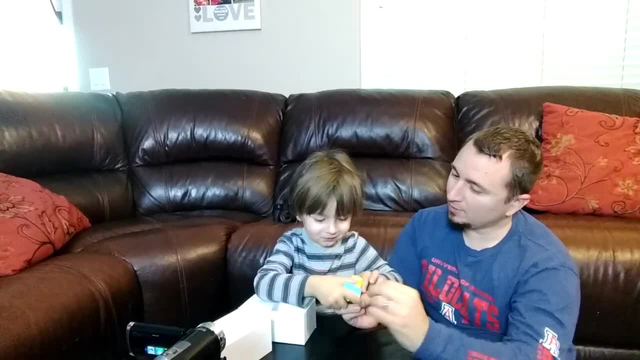 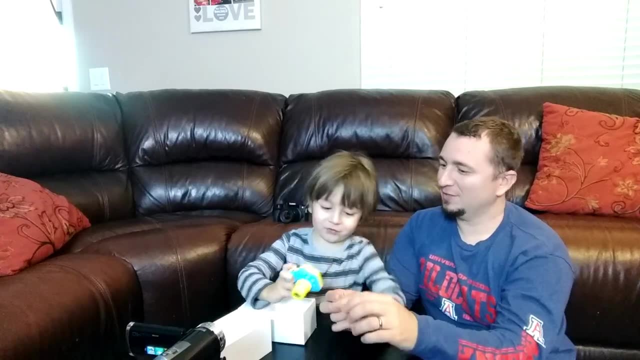 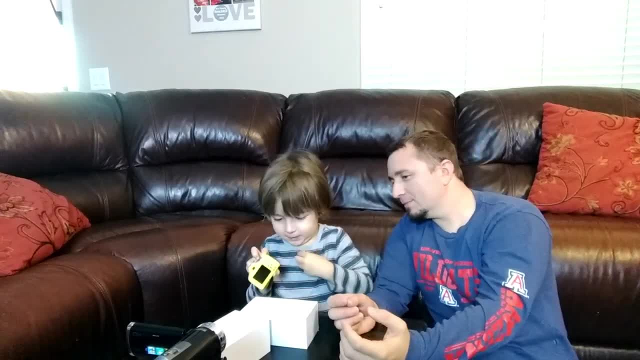 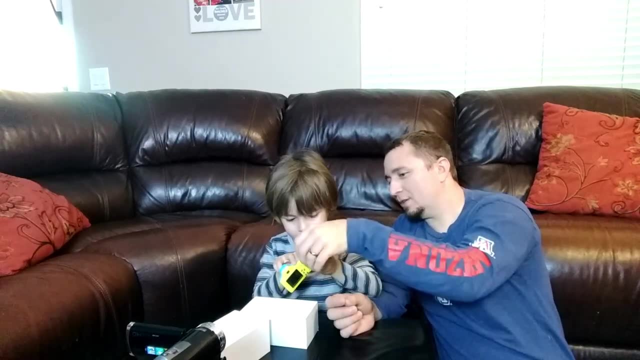 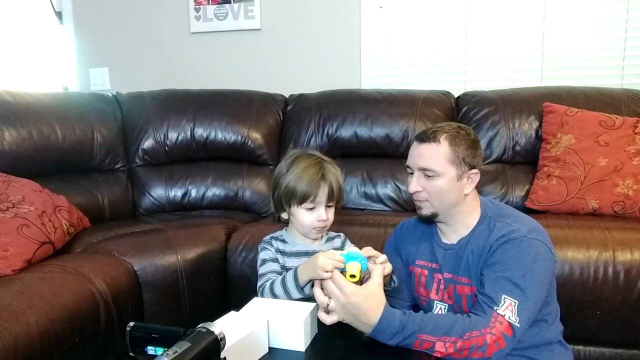 Yeah, This way, like this. Let's see, Maybe that way. Okay, Like this. Okay, so the memory card goes right here. Okay, Oh, that's your little screen, So how are you going to turn it on? 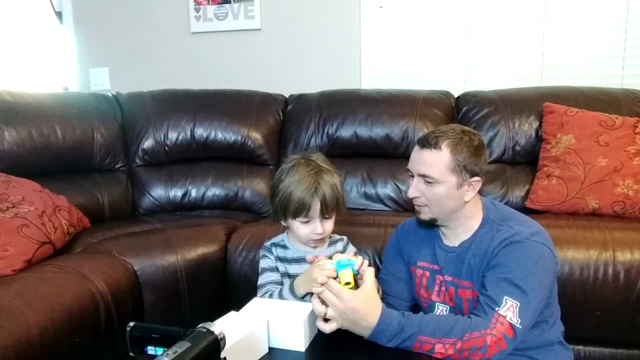 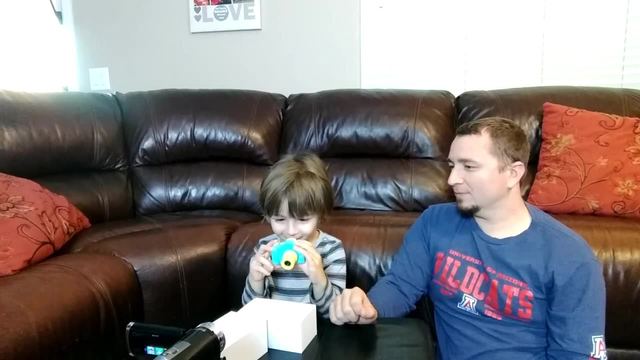 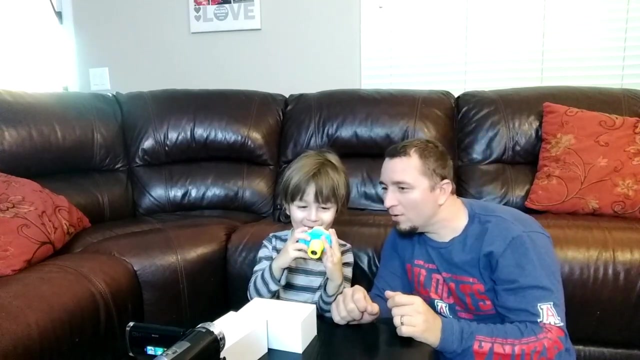 To turn it on. it's a little power plug. See how the little button right here- This one, Yeah, It says welcome, Okay, Oh, Can you take a picture? Yeah, Just right there, top right. Okay, Whoa, So we can take a picture. This is four gigabytes. Remember the keys? 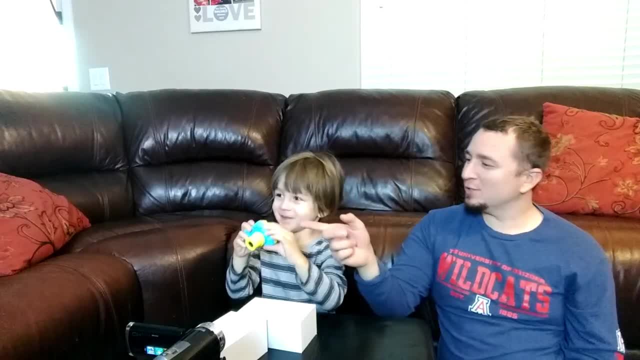 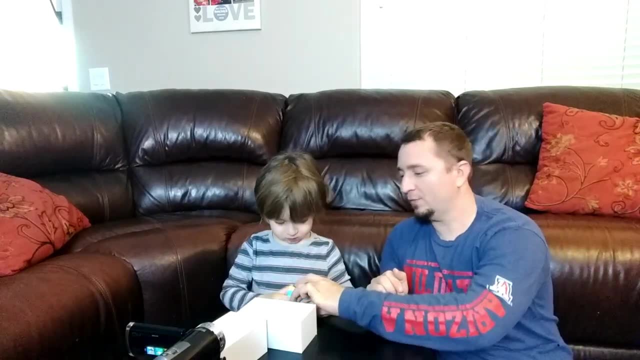 Look it, Whoa. So this is a four gigabyte car. This is a four gigabyte car and it takes about 1,500 pictures. it shows on there. So we take a picture. it holds it for let's see. can you show the camera? 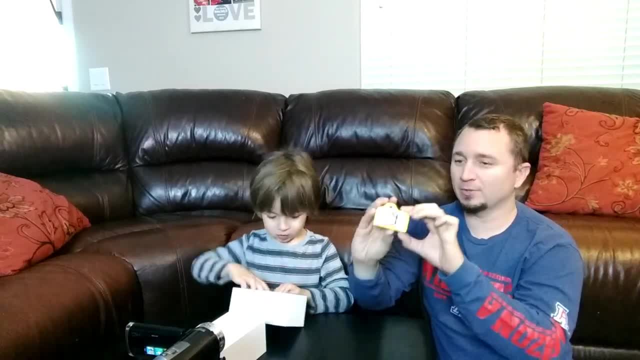 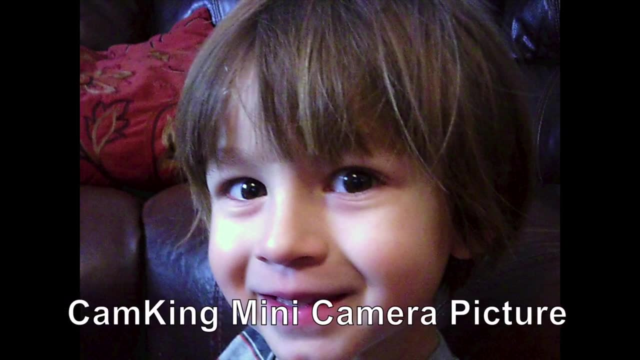 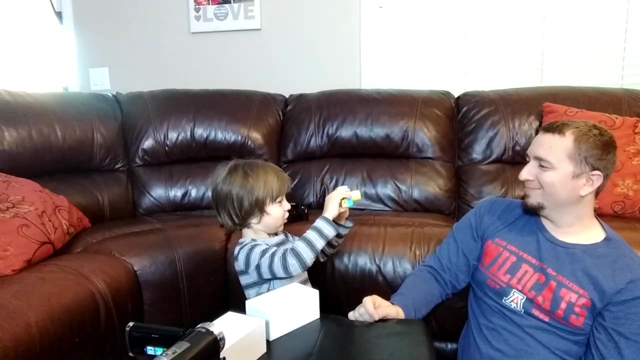 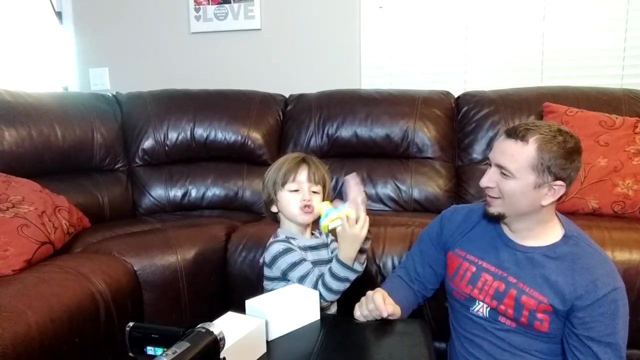 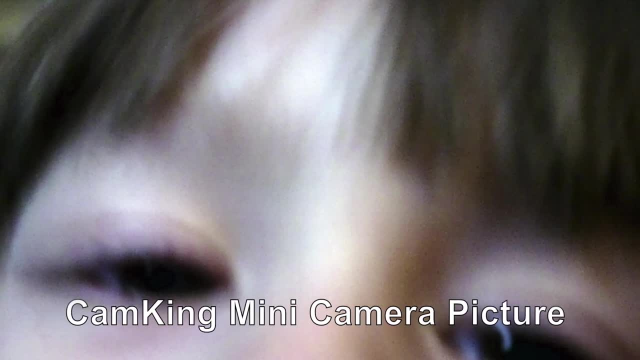 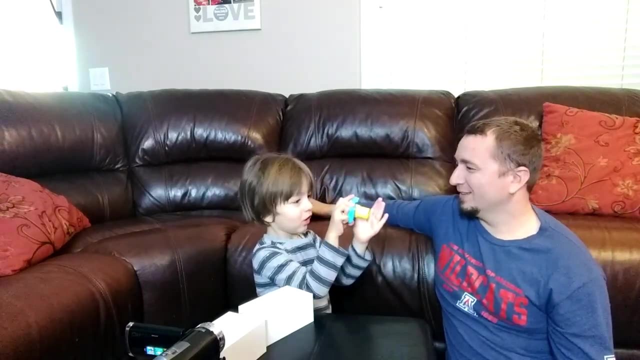 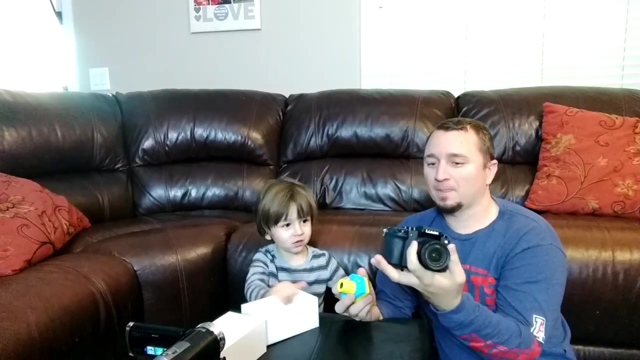 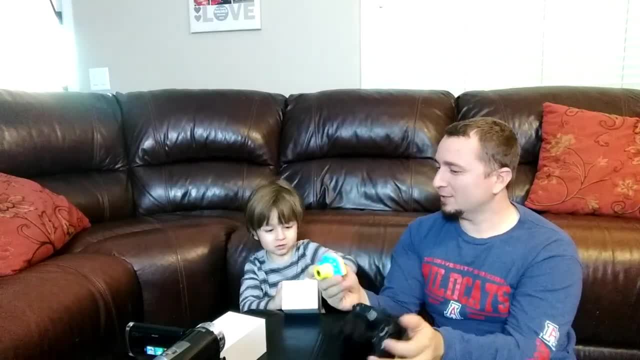 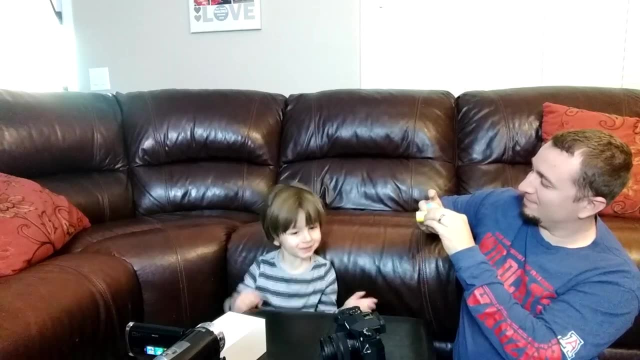 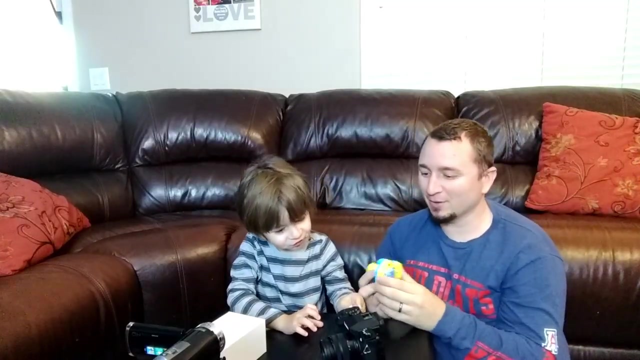 This is a Micro Micro, A good micro micro camera. Eli likes it. It has a cool power button. you can take a picture, cheese. We'll see how the pictures look once we put it on the computer And it looks just like daddy's little camera. 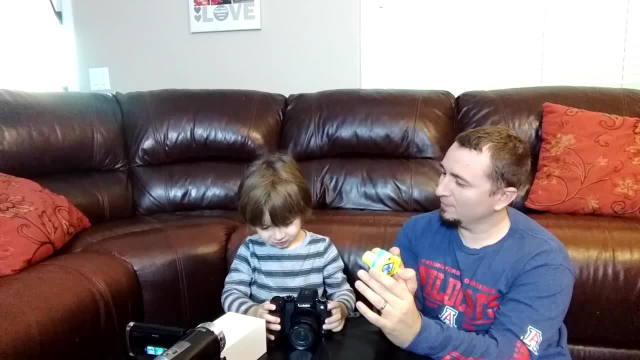 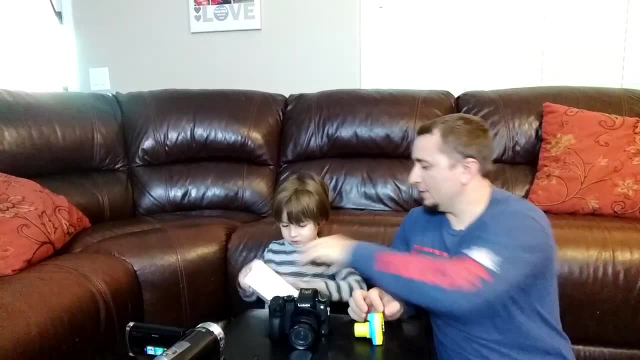 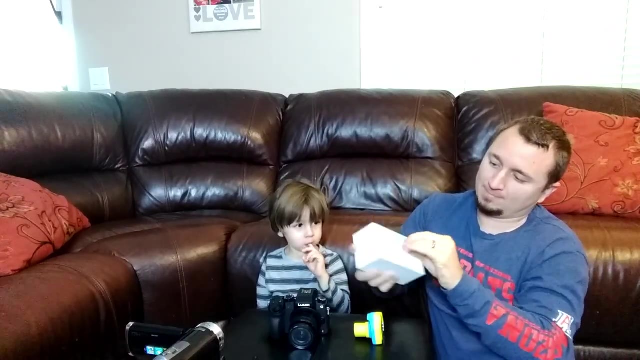 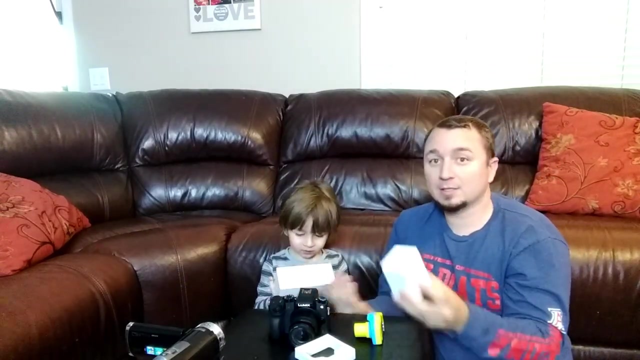 It's just basic point and click photography. You like it? Yeah, So what else comes in the box? So in the box we have, let's see what do we have here? you got stickers. he had stickers, so he could go ahead and put it on his camera. if he wants to put more stickers on there, 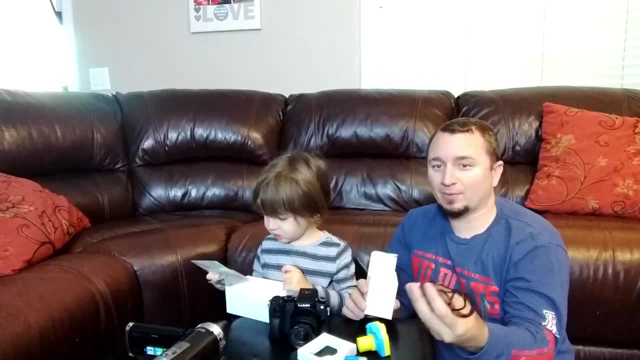 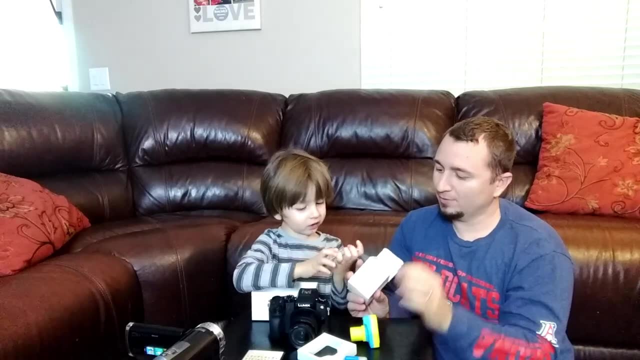 You get your USB charging cable, which I went ahead and charged this ahead of time. it comes not fully charged, so you want to go ahead and charge it before you give it to your little kid, Okay, And then we have a little lanyard. oh, look at this. 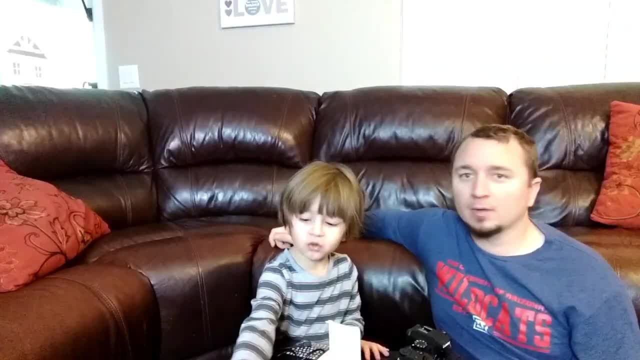 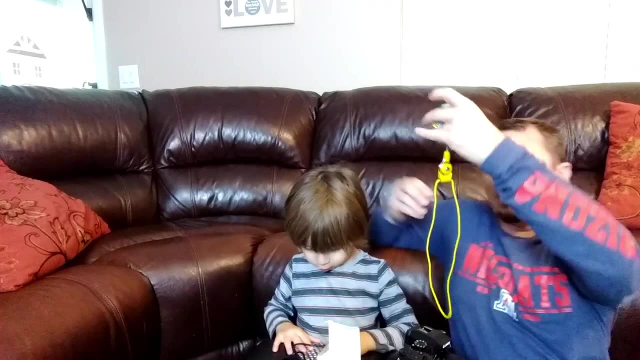 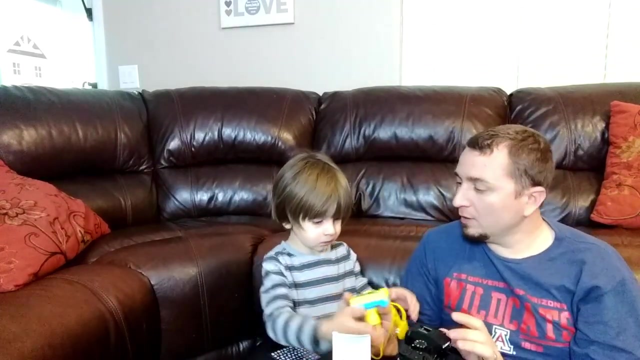 So we can go ahead and put it right here. So we put the little lanyard on his camera, so he could go ahead and take this off if he wants to, Or you can put it back on. Eli, you know what we should do. 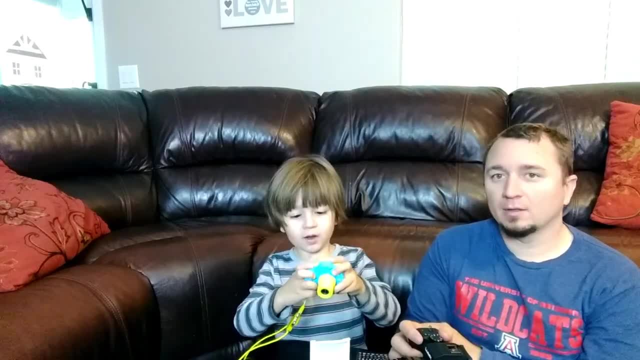 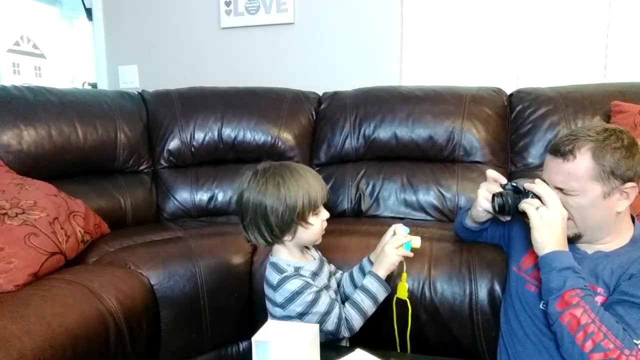 We should do a side by side comparison of a photo. So Eli's going to turn his camera on and take a picture. 1, 2, 3, 2.. Ready- 1,, 2,, 3, 2.. 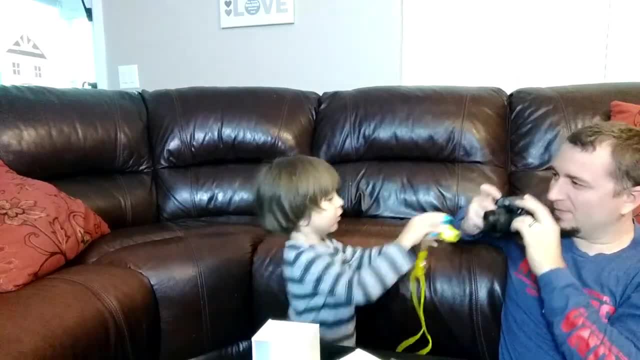 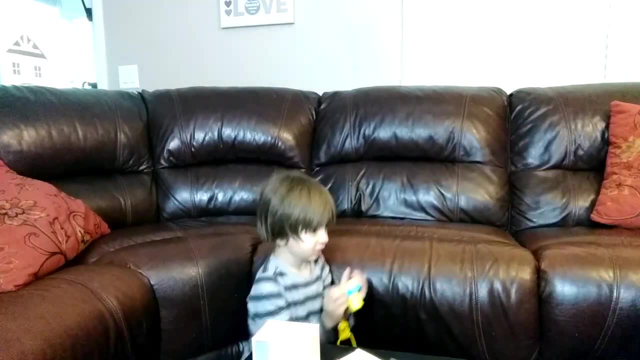 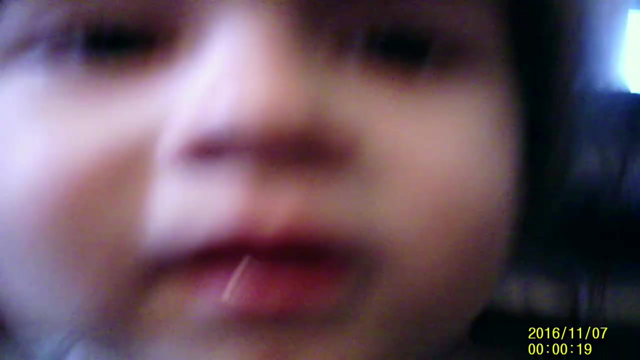 Okay, Again ready. 1,, 2,, 3,, 2.. It's recording video, So tell me something. So this is the video that Eli's recording off his little camera. So this is Eli's camera, Yeah, 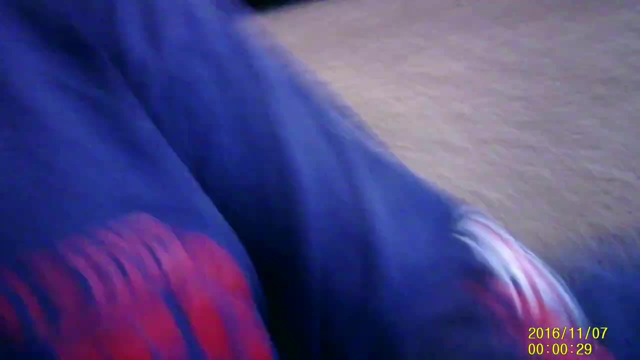 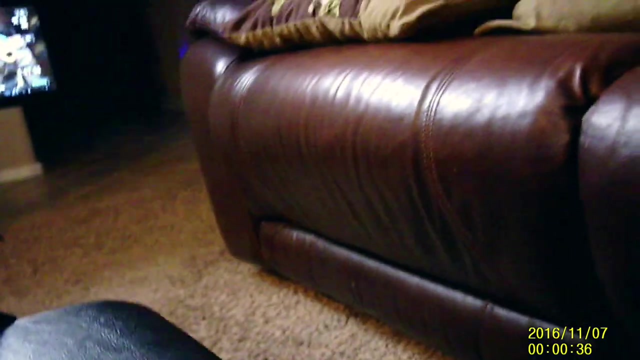 And so we're going to see the quality. Did it show record? Oh nice, look at this. It's recording. So you want to hold it down for a couple seconds Here. So it's constantly recording. So you turn it off.